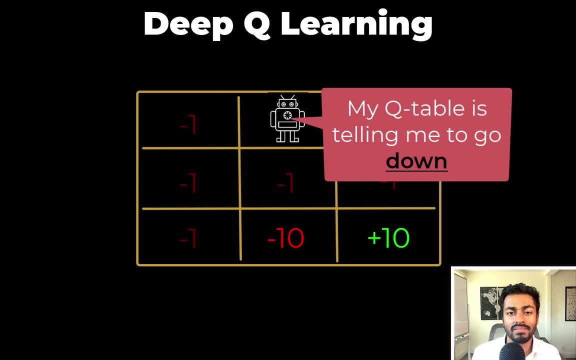 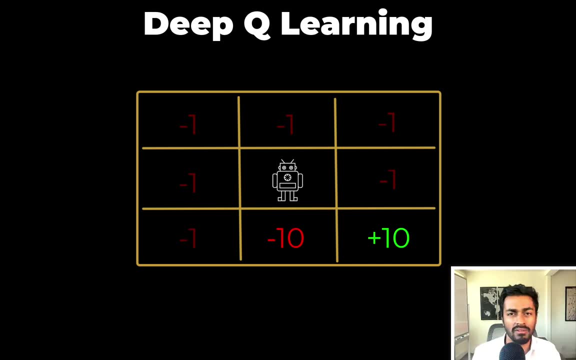 what about now? My Q-table is telling me to go down. You go for it, buddy. Now, this is a simple world of just nine grid squares, where there's a finite number of states. but what if there were a lot of states? Well, that would mean that this Q-table 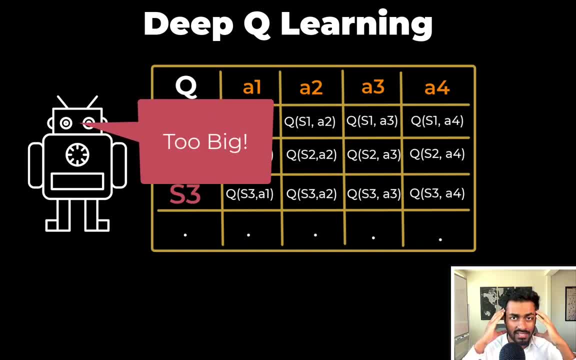 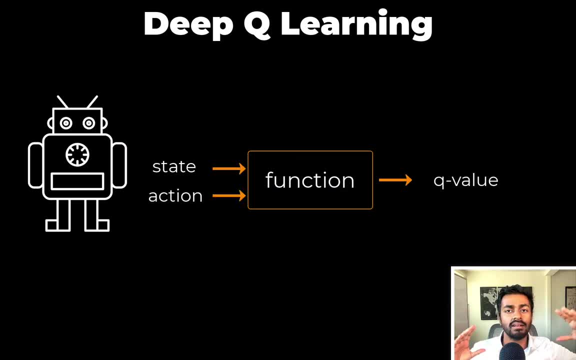 becomes really big, too big to fit in Frank's tiny little head. It would literally run out of memory. So instead of having this table as a conscience, it's probably better to just have a function as Frank's conscience, And this function would just take in a state and an action and it would output some value that 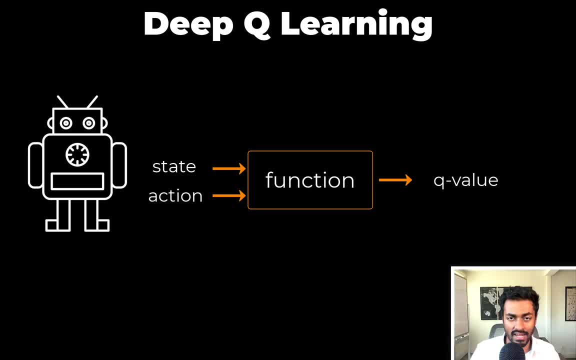 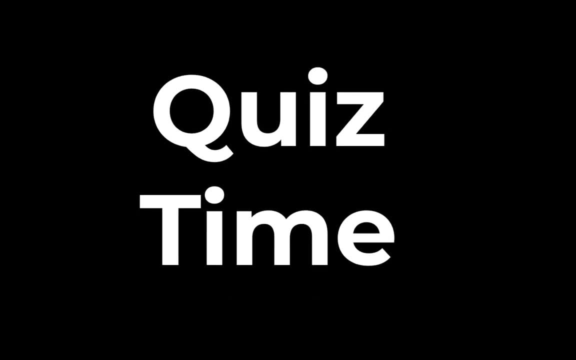 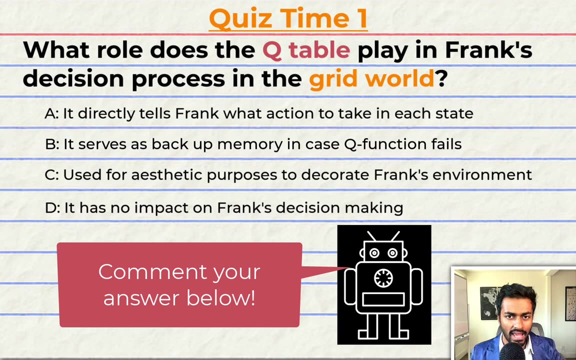 emphasizes how good that action was taken for the state. This value is known as a Q-value. by the way, Quiz time. Have you been paying attention? Let's quiz you to find out: What role does the Q-table play in Frank's decision process in the simplified world of nine squares? 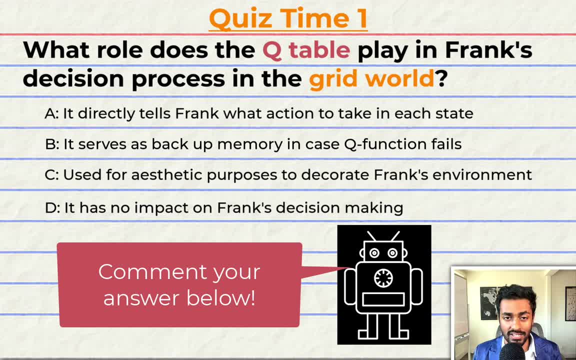 It directly tells Frank what action to take in each state. It serves as a backup memory for Frank in case the Q-function fails. It's used for aesthetic purposes, to decorate Frank's environment Or D. It has no impact on Frank's decision making and he relies solely on the 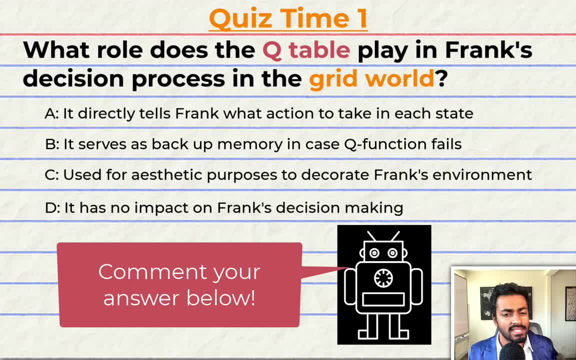 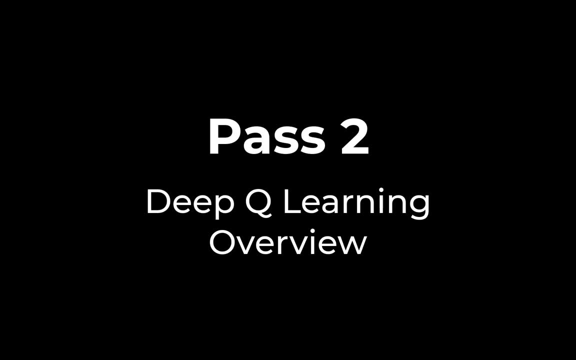 Q-function. Comment your answer down below and let's have a discussion Now. at this point, if you think I deserve it and you like, Frank, please do consider hitting that like button. That'll do it for quiz time for now, but keep paying attention because I'll be back again. 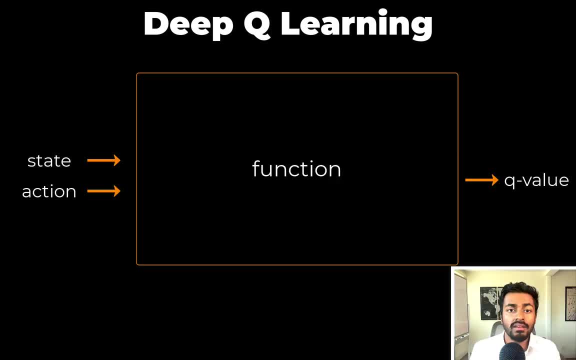 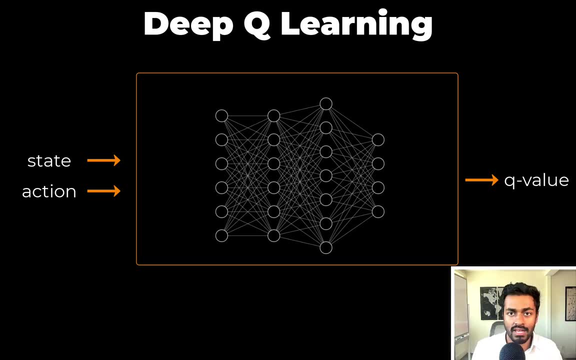 So we replaced this giant Q-table with a function. In the context of AI, this function is typically a neural network, So Q-learning is to learn values in a Q-table. Deep Q-learning is used to learn the parameters of a Q-network or a neural network. 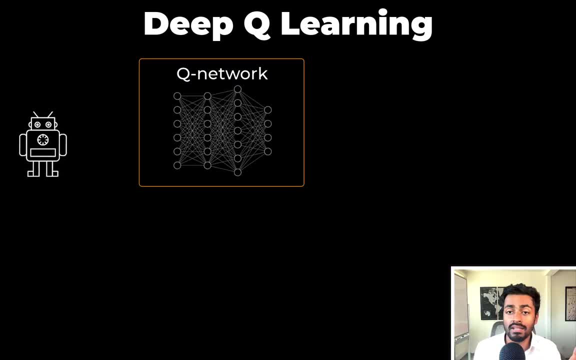 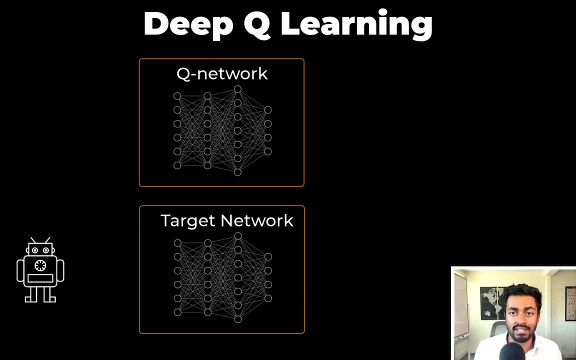 Now, this Q-network is randomly initialized and represents Frank's conscience. We have a target network that represents the ideal conscience, and this is the same architecture as the Q-network. The goal now is to compare Frank's current conscience with Frank's ideal conscience And from this comparison we can compare them, get a loss and use this loss. 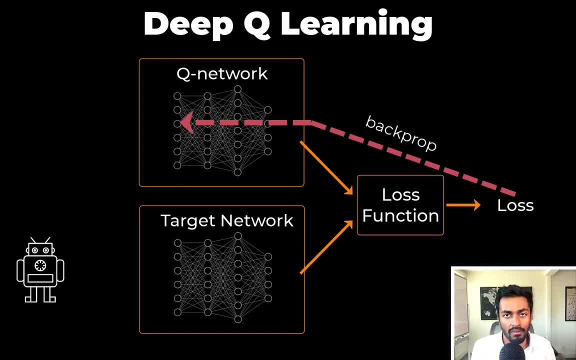 as an example. Now let's take a look at the Q-network. First let's create the parameters in the Q-network with backpropagation, And then the cycle repeats. In the next pass we're going to get into more details, but for now in 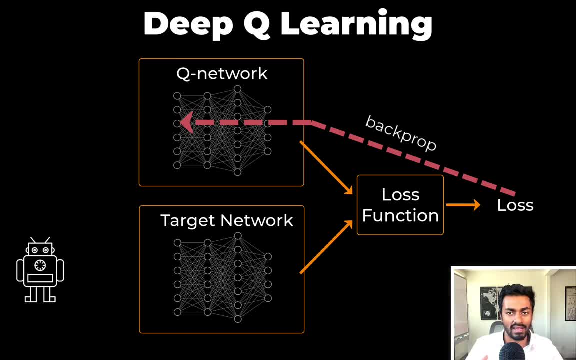 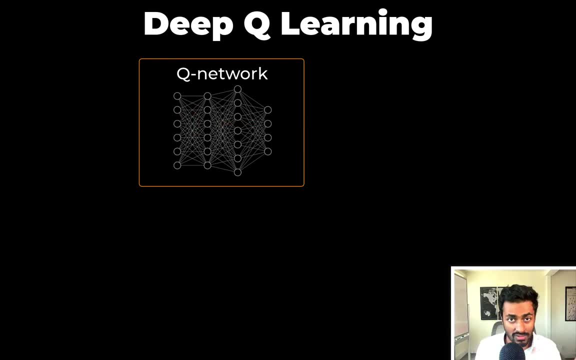 order to train this network, we actually first need to take a step back and collect this data. So let's just talk about that very briefly. So this data collection, first of all, is done using this Q-network. It's first randomly initialized and some state is chosen. The 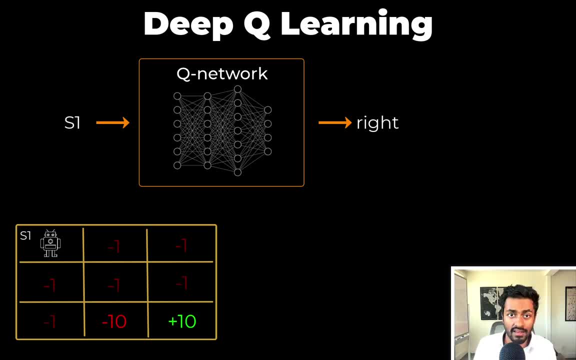 Q-network will generate the data. It will generate the action to take. This action is taken And then a reward is gained and the agent goes to the next state. So the quadruple of the state, the action, the reward and the next state is then taken and stored in some memory called the experience replay. 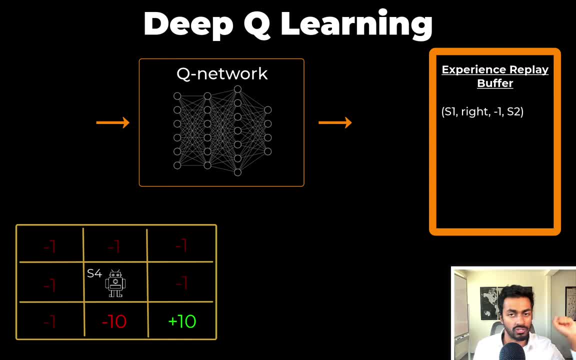 buffer And we repeat this process of just choosing some state producing these quadruples and storing them. So this data is now in our experience replay and then can be later used to train our Q-network, which we just discussed before Quiz time. 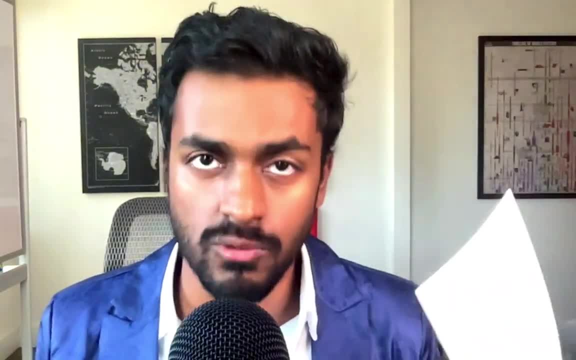 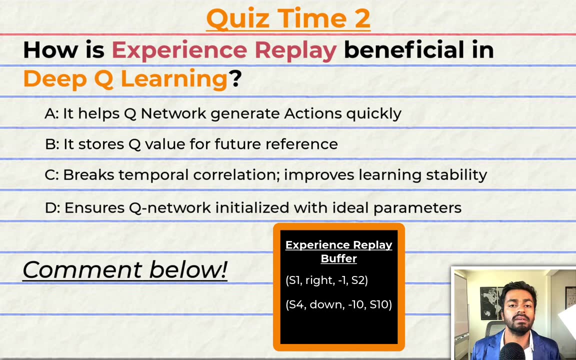 It's that time of video again. Have you been paying attention? Let's quiz you to find out. Why is experience replay considered beneficial in deep Q-learning? A- it helps the Q-network generate actions more quickly. B- it stores the Q-values for future reference. 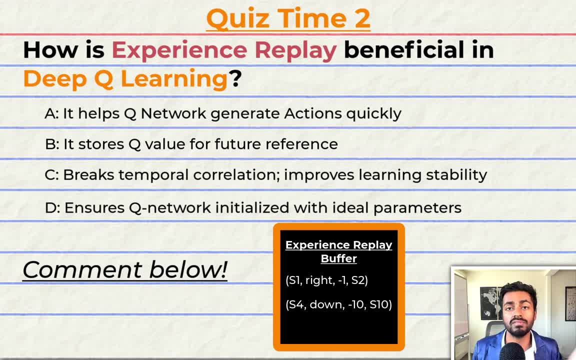 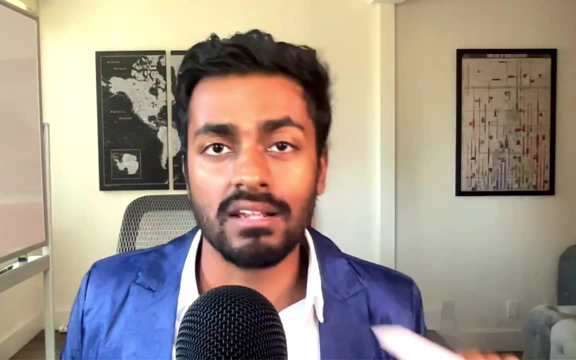 C, it breaks the temporal correlation and improves learning stability. Or D, it ensures that the Q-network is always initialized with the ideal parameters. Comment your answer down below and let's have a discussion. That'll do it for quiz time for now, but once again I will be back, so pay attention. 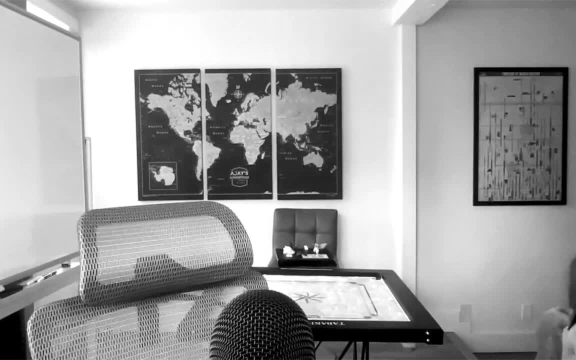 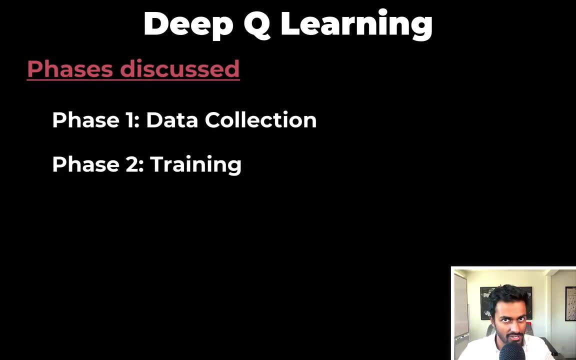 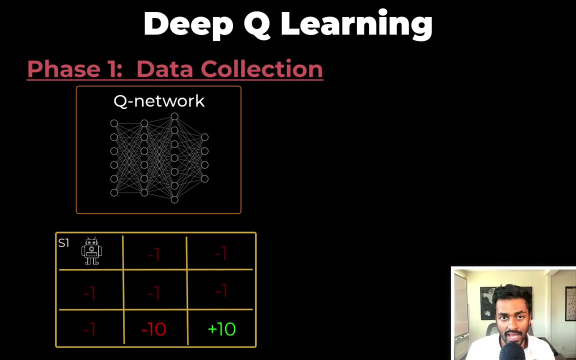 Now there are two phases that we discussed in pass 2.. That is the data collection phase and the training phase. So let's talk about both in detail, Starting with the data collection phase. So first we randomly initialize the Q-network. We choose an initial state, Pass it through. 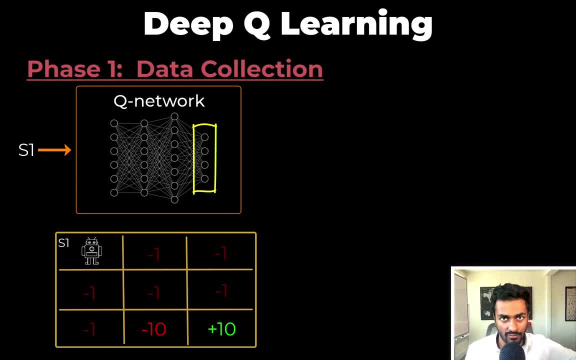 the Q-network, And the number of neurons, by the way, is the number of neurons in the data collection phase. The number of neurons, by the way, in the output layer of this network is the number of possible actions. So each neuron outputs a Q-value for the input state at a specific action. 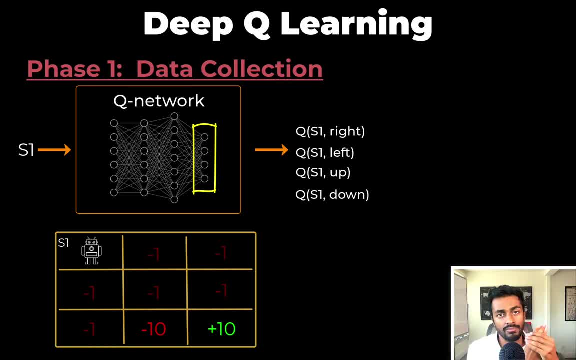 So, for example, if we could only go left, right, up or down, there would be four neurons in the output layer And each of these neurons would correspond to a Q-value for each of those actions. So we then choose an action in an epsilon-greedy fashion. 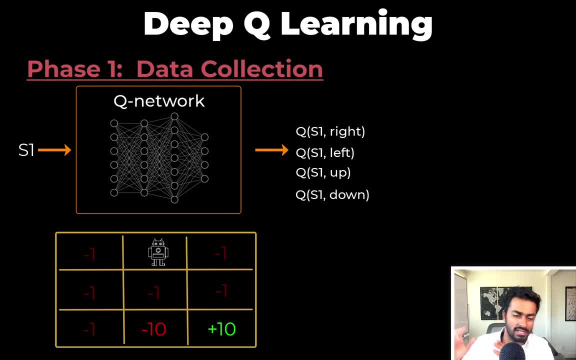 We take the action in the environment or in some simulated environment, And once the action is taken, Frank will get a reward and Frank will also be in a new state. So now we take that quadruple that we just described. that is, the state, the action. 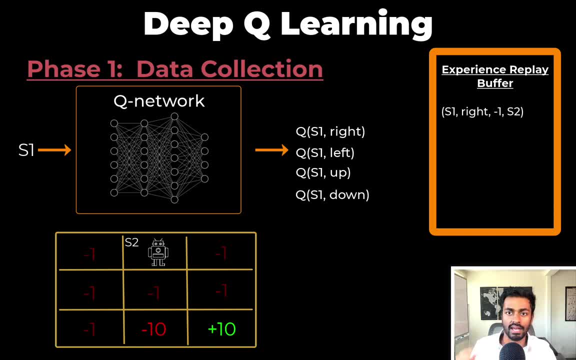 the reward and new state and store it into the experience replay buffer. Now we can randomly choose a new state and repeat the process of collecting the data in the experience replay buffer. And this is the data collection piece. Now onto training. Now we have this experience replay, which has a lot of data. 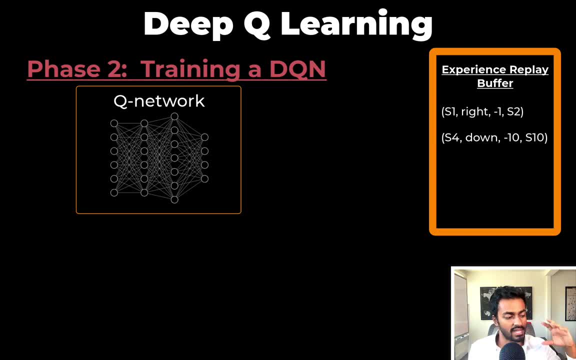 And we can use this data to train the Q-network. So let's take a batch of this data Now. in this case, just for explanatory purposes, let's say the batch size is just one example, so that we can see what's going on throughout. 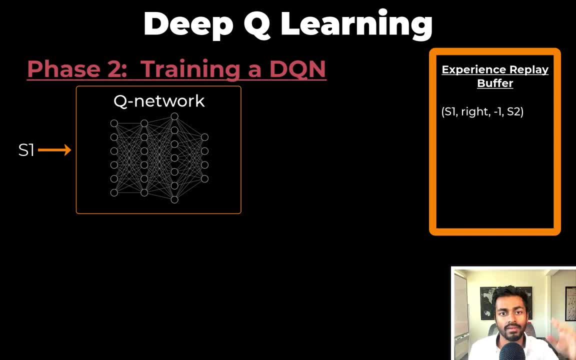 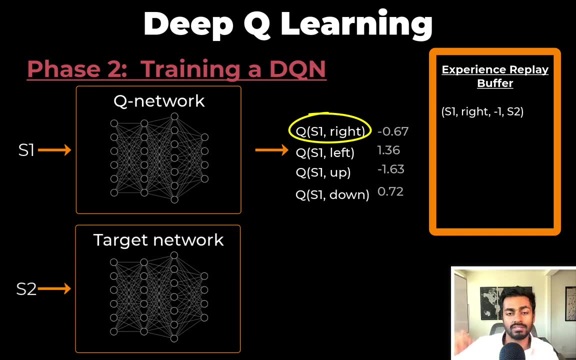 We feed the current state of the quadruple into the Q-network. Okay, We get the Q-value corresponding to the action in the quadruple And then we also take the same current state, pass it through the target network and we get the highest Q-value there. 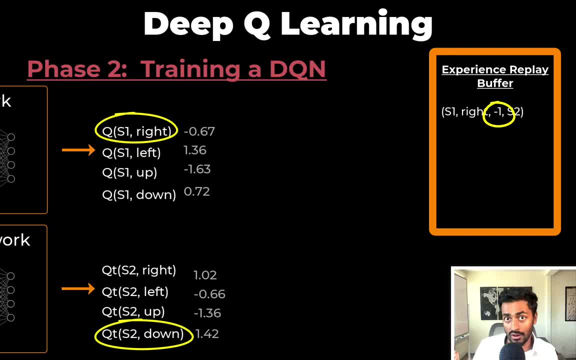 Now we take the reward from the quadruple and add it to this target Q-value. So now we have two main values: one from the target- It's an ideal Q-value- And then we have the current Q-value. Now we're going to compute the mean squared loss. 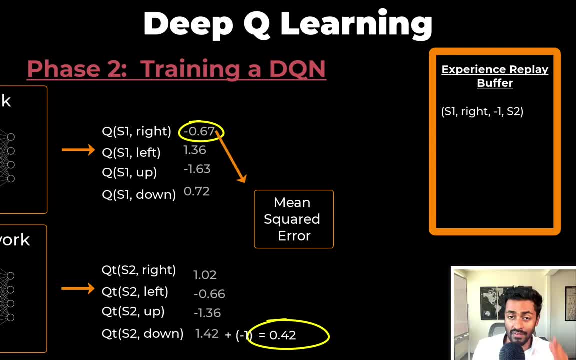 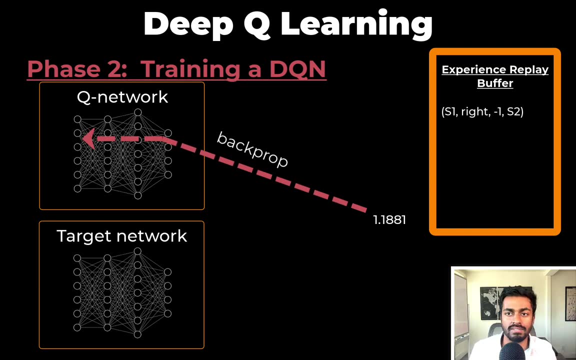 Using the Q-network's Q-value that represents Frank's conscience and the target final Q-value that represents the optimal decision. This loss is then back-propagated into the Q-network and the parameters are updated. So Frank learns, but the target network remains the same. 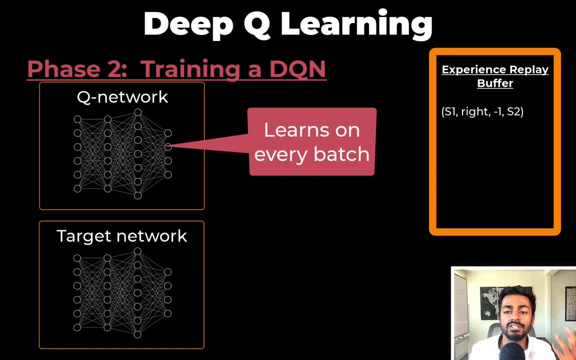 Now we repeat the process for a few batches, where Frank's conscience continues to learn, but the target network still remains the same. And then, after a few batches, we will update the parameters of the target network to then match the Q-network, and then continue. 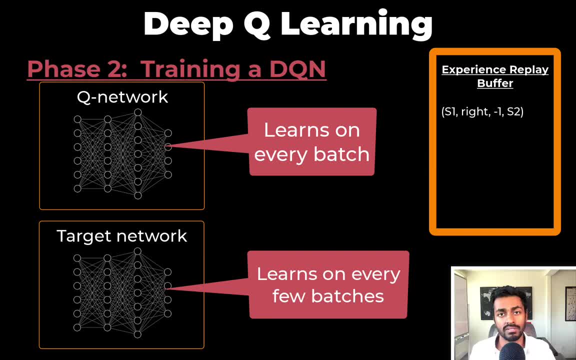 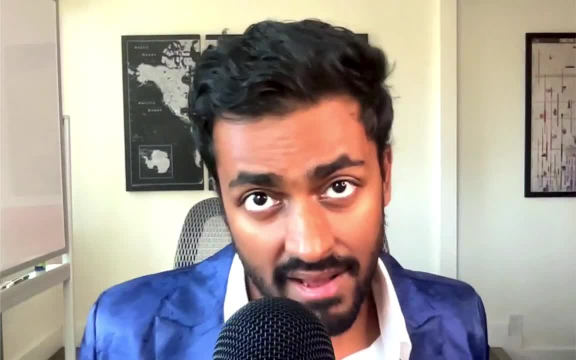 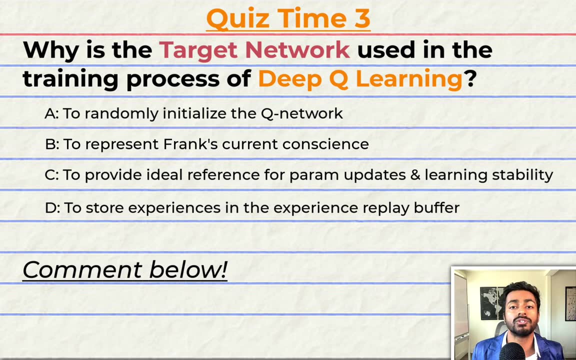 And eventually Frank's conscience and decision-making improves. and he's a champ Quiz time. I'm back. Have you been paying attention? Let's quiz you to find out. Why is the target network used in the training process of deep Q-learning? 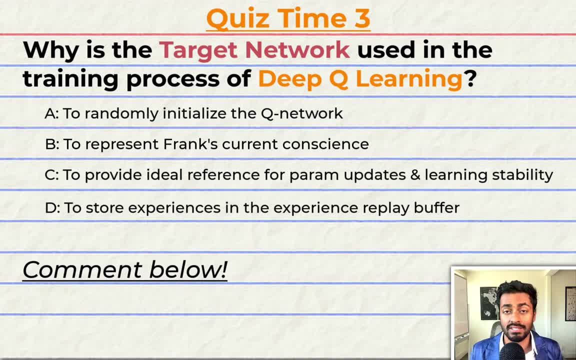 A- The Q-network. B- The Q-network. C. To randomly initialize the Q-network. D. To represent Frank's current conscience. C- To provide an ideal reference for parameter updates and improve learning stability. D- To store experiences in the experience replay buffer. 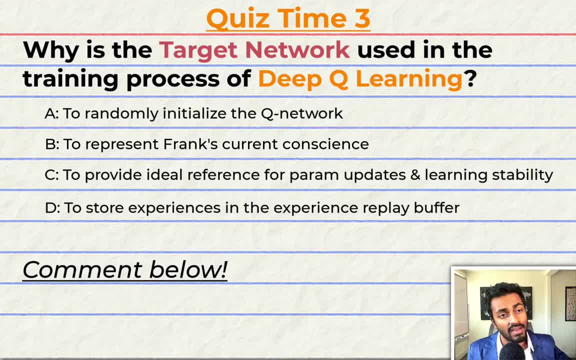 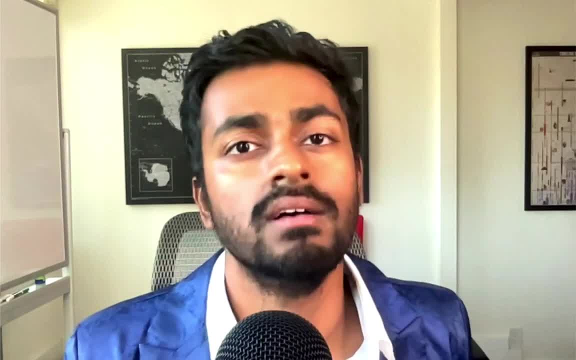 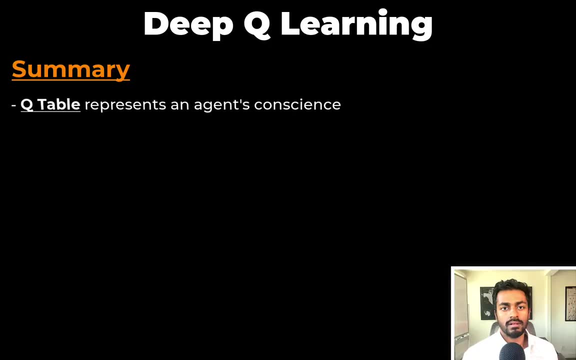 Comment your answer down below and let's have a discussion. That will do for quiz time for now And unfortunately I'm not going to be back again, So before we go let's get a summary of the video. A Q-table represents an agent's conscience. 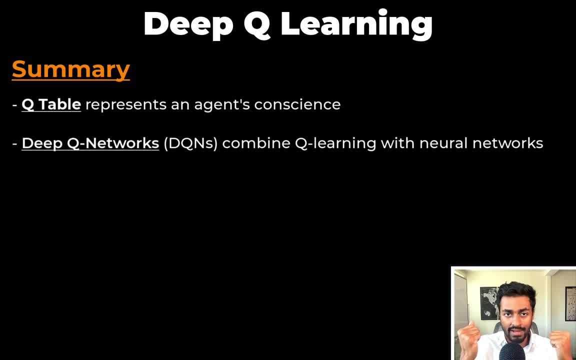 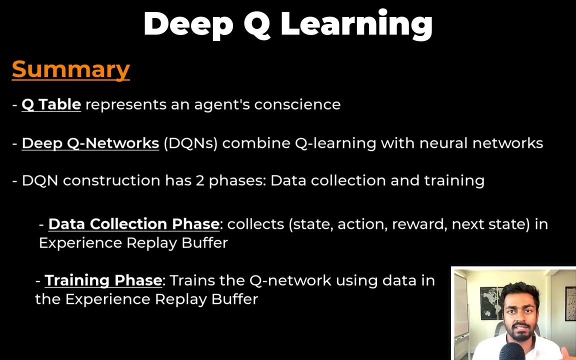 The deep Q-networks combine Q-learning with neural networks. DQN construction has two phases: a data collection phase and a training phase. The data collection collects independent quadruples of experiences in data stores called the Experience Replay Buffer, And the training phase trains the Q-network using data in this Experience Replay Buffer. 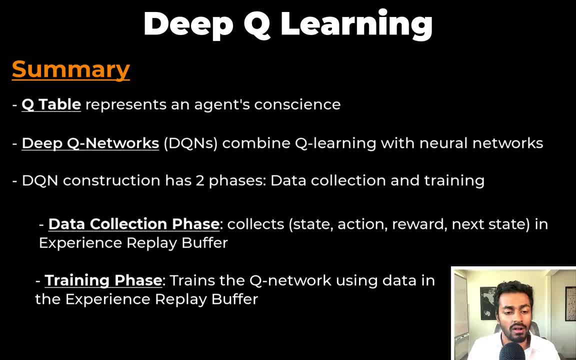 And that's all we have for today, But if you want to know information more about the raw Q-learning algorithm, do check out my video right on screen here And, as always, thank you all so much for watching. Please consider liking the video. 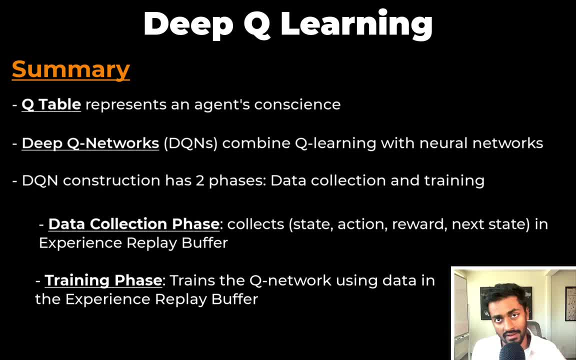 If you do think I deserve it, And I will see you in the next one. Bye-bye.